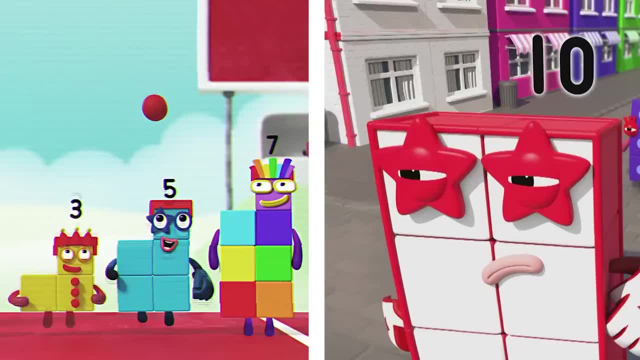 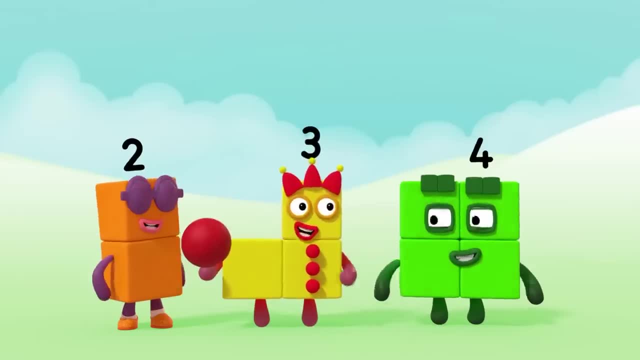 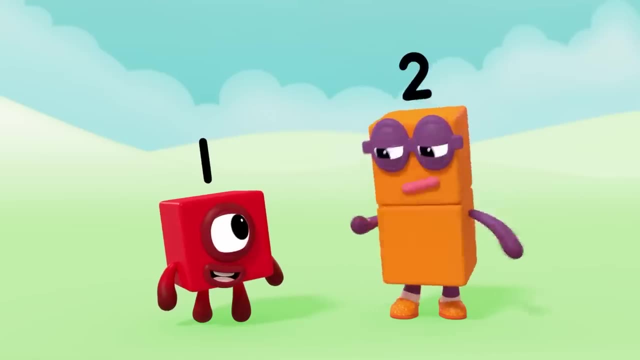 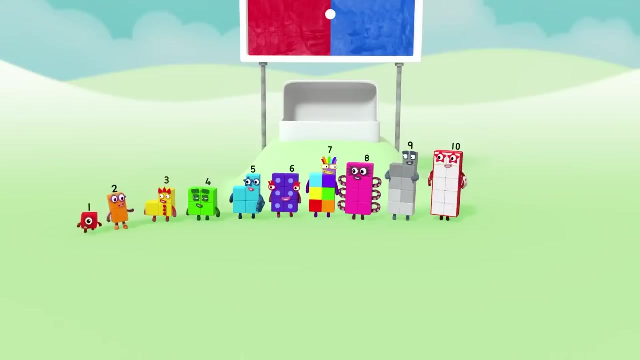 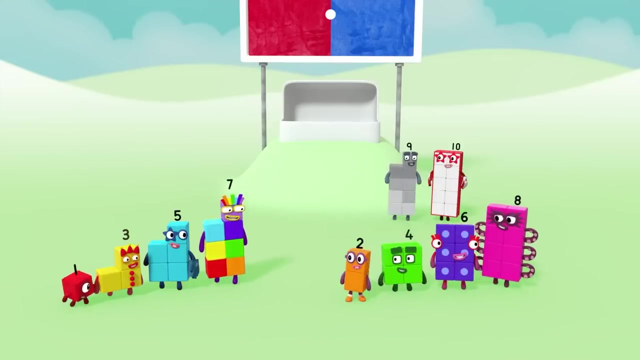 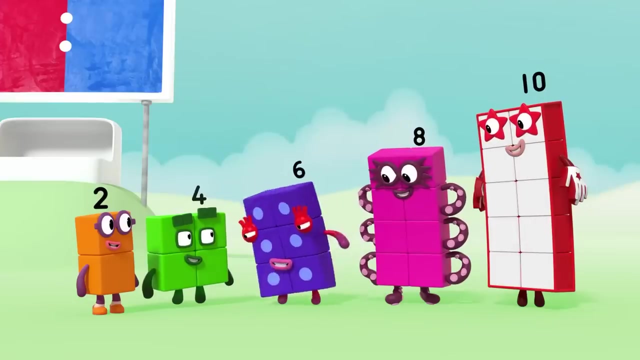 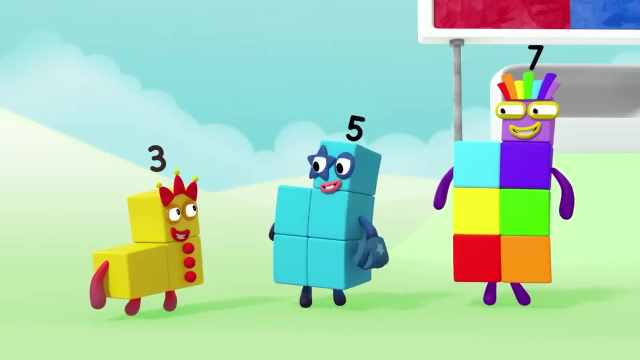 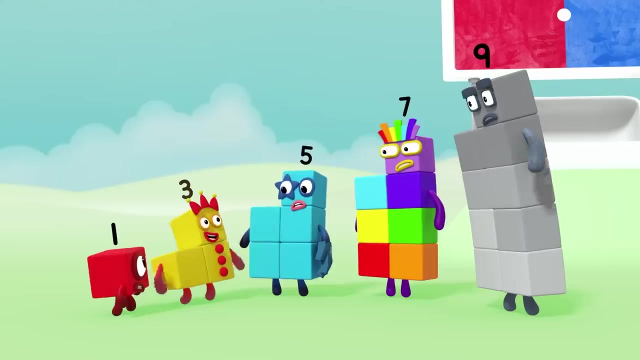 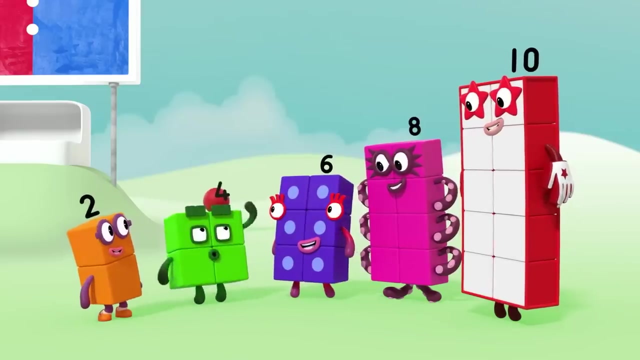 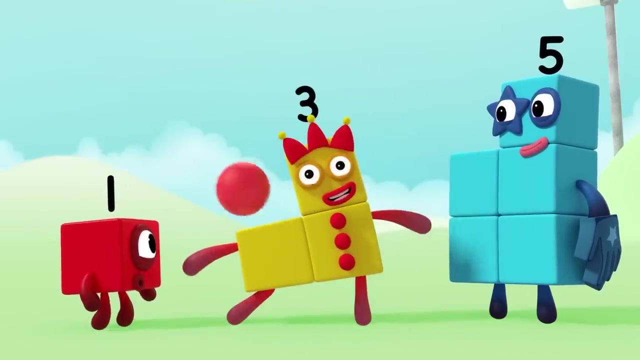 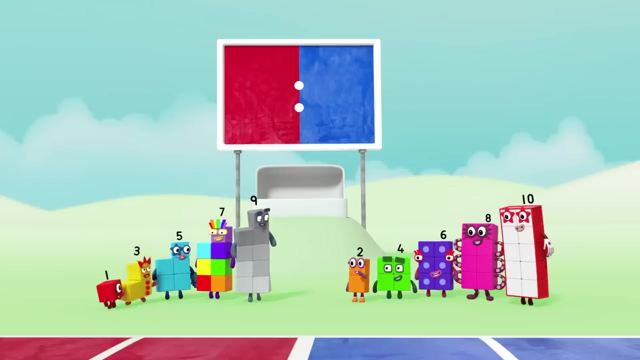 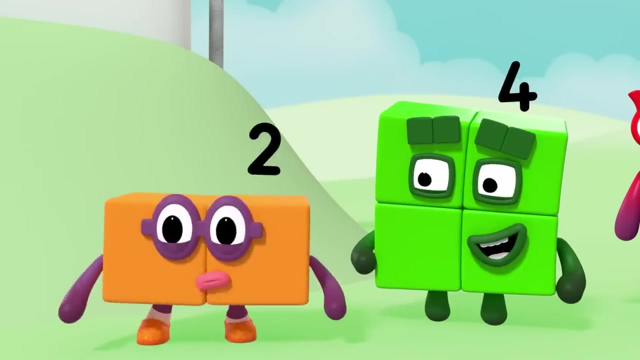 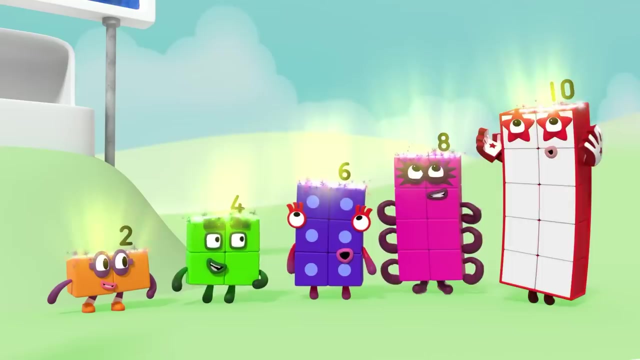 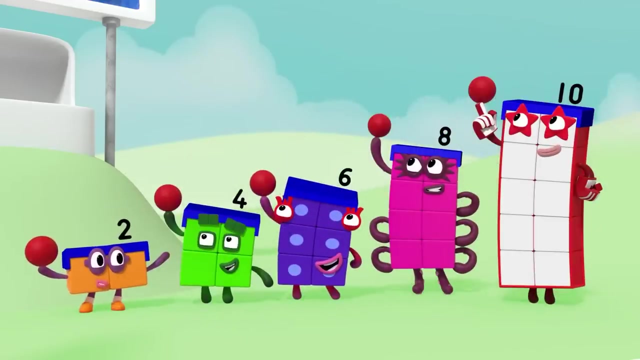 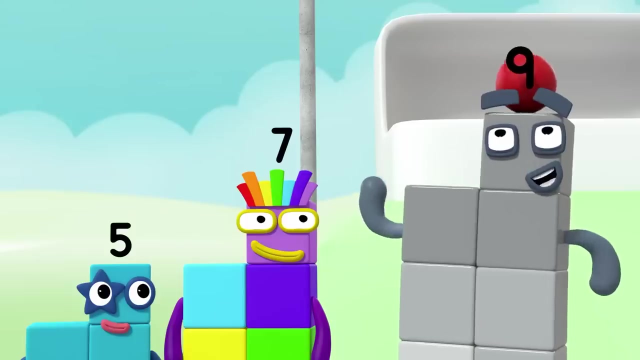 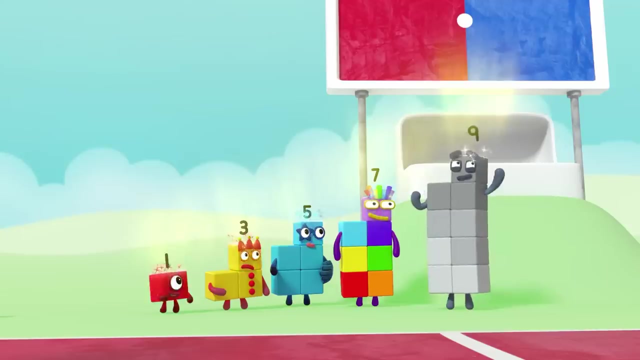 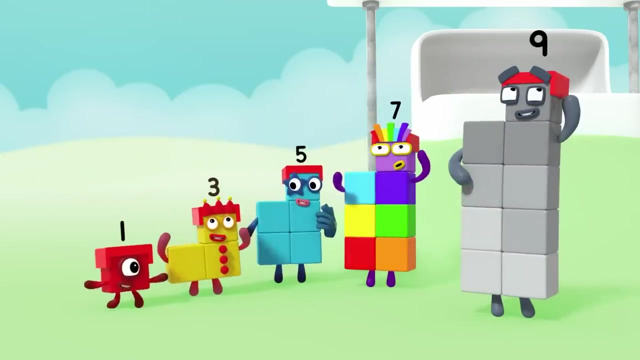 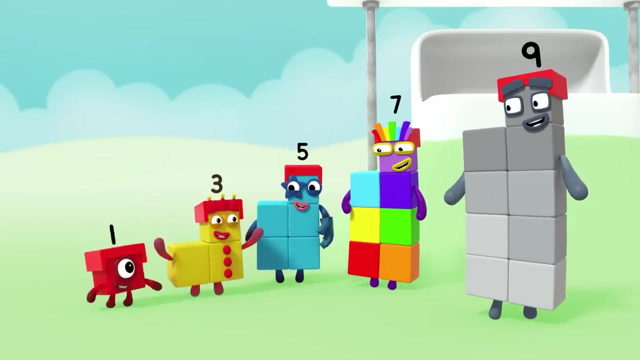 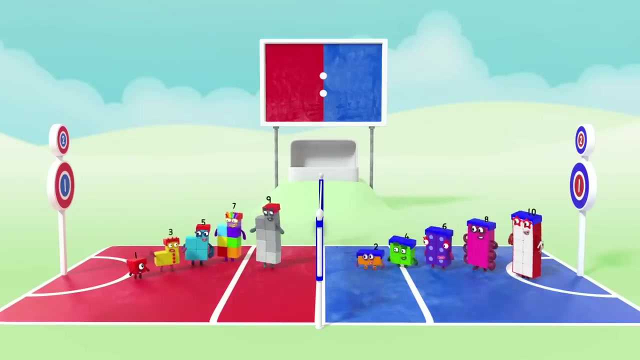 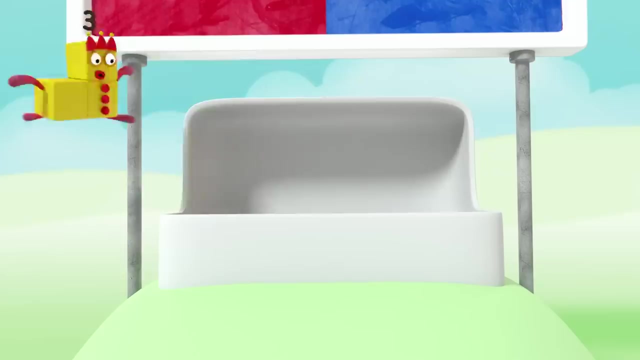 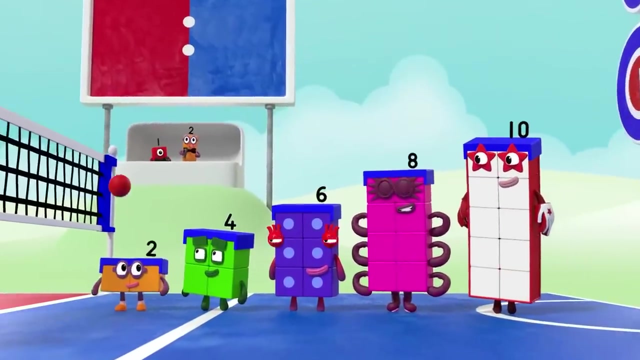 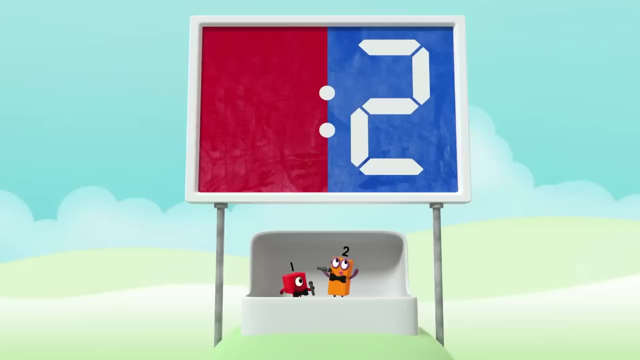 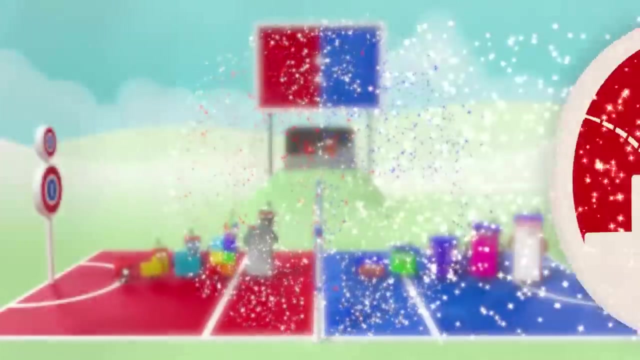 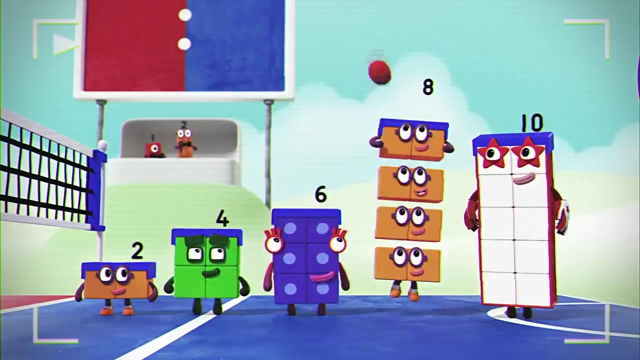 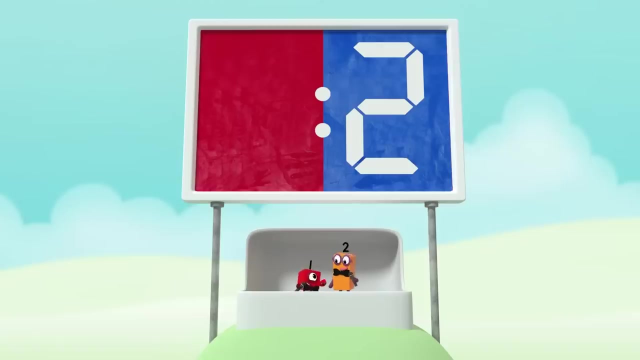 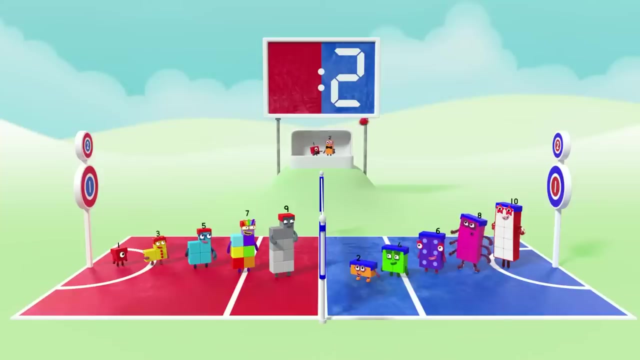 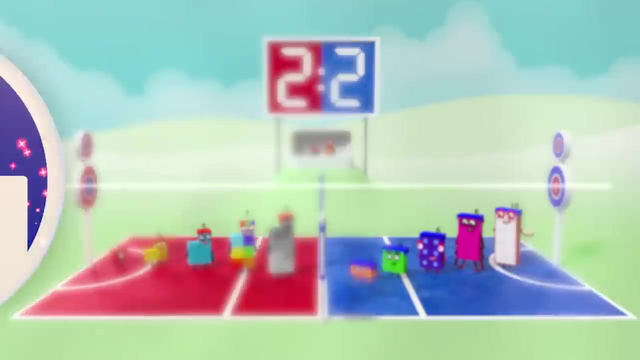 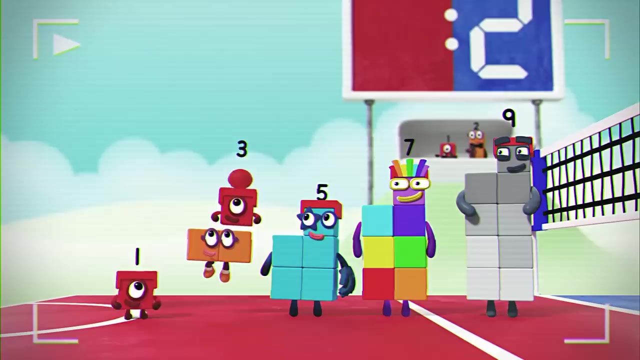 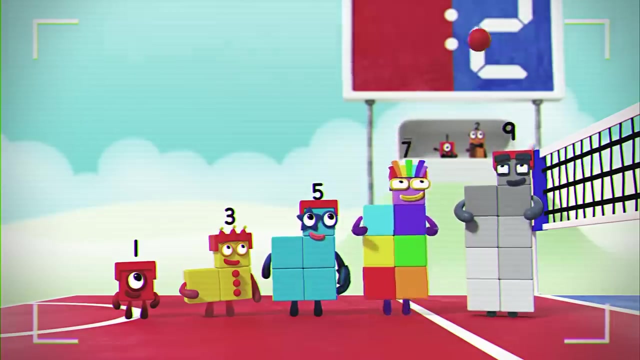 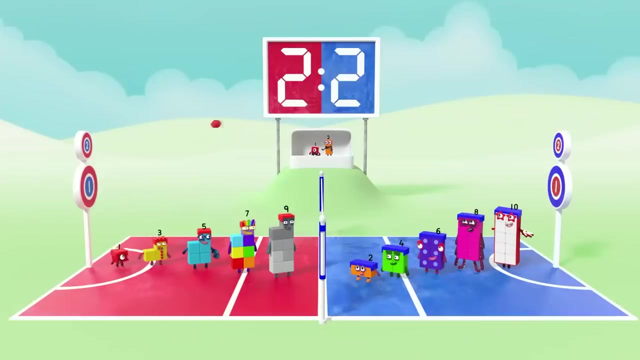 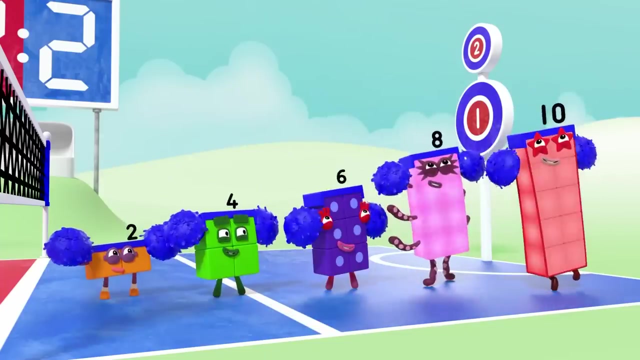 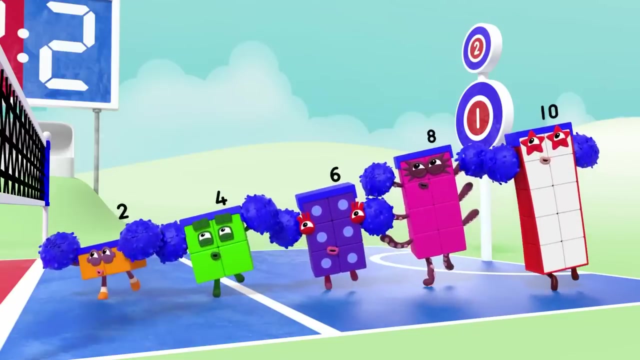 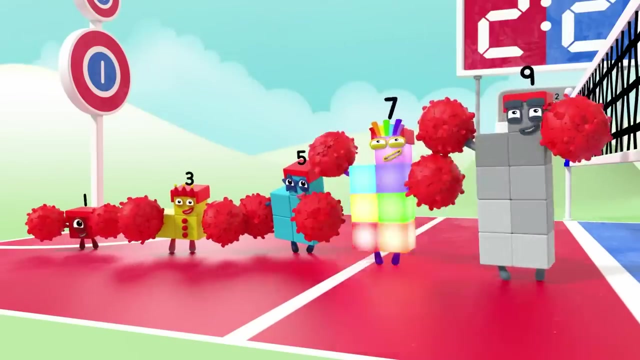 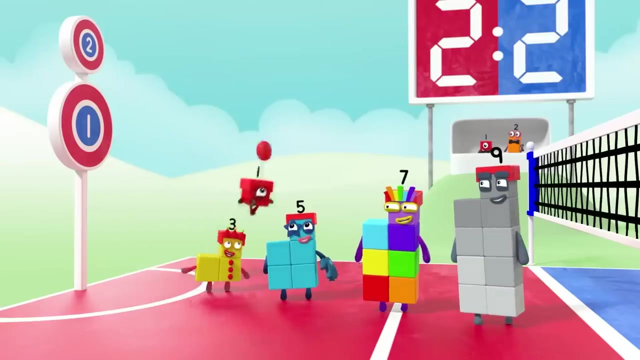 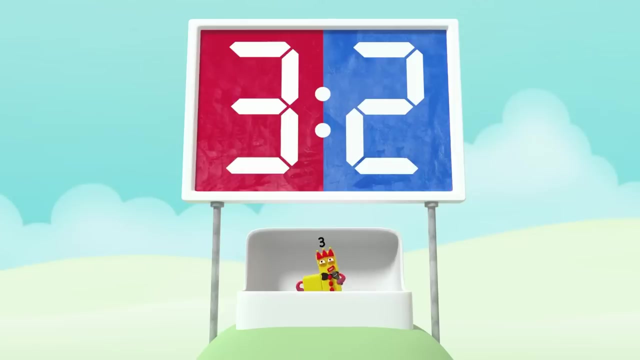 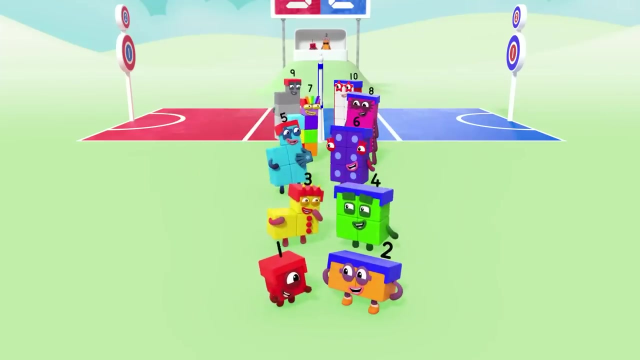 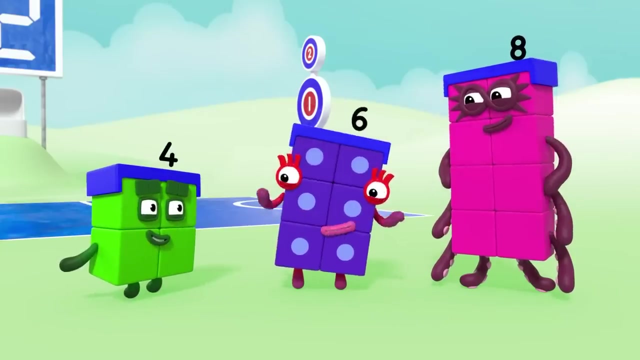 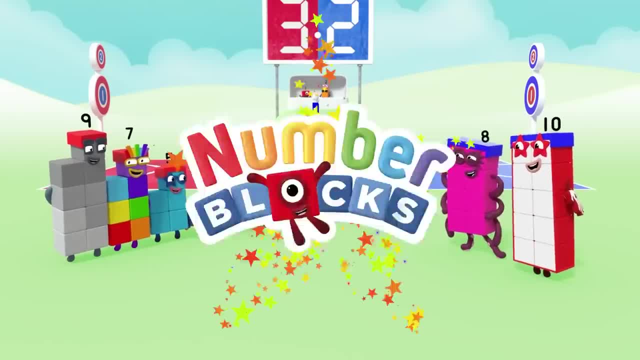 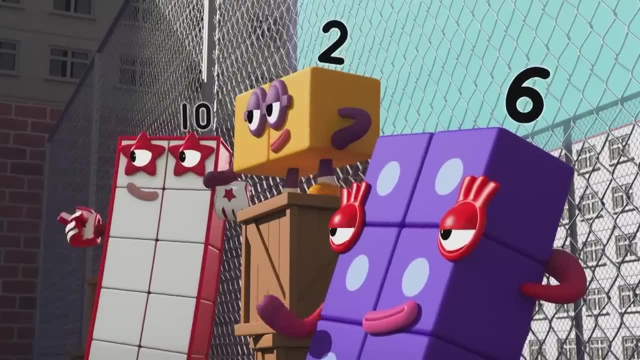 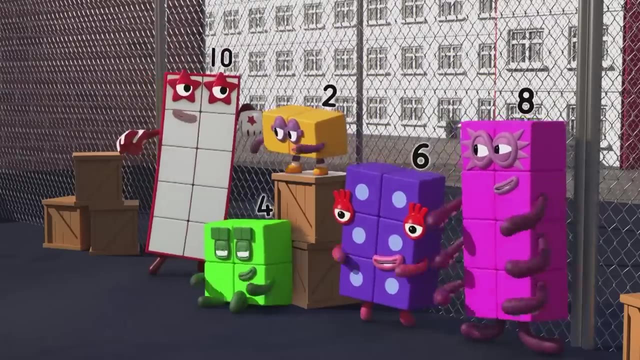 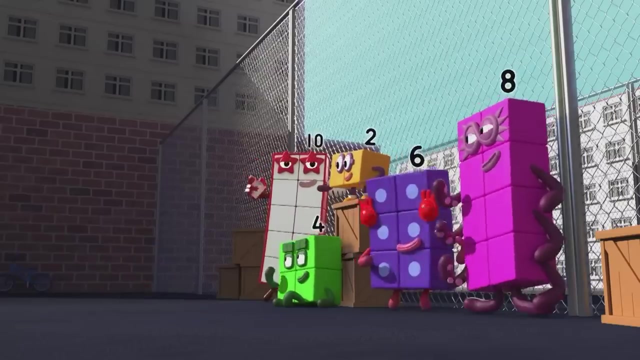 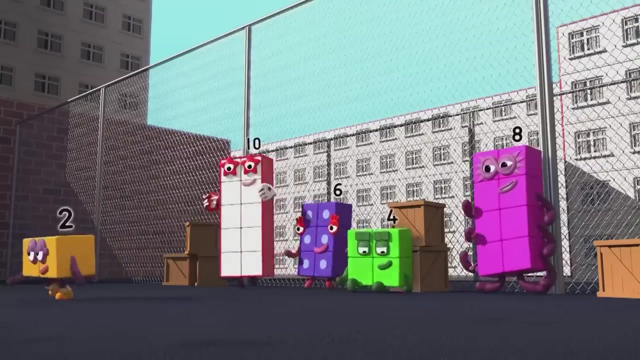 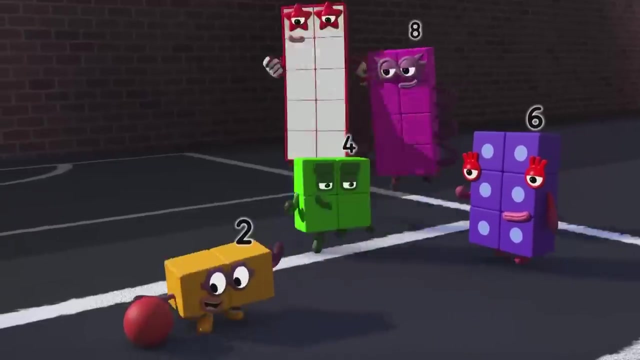 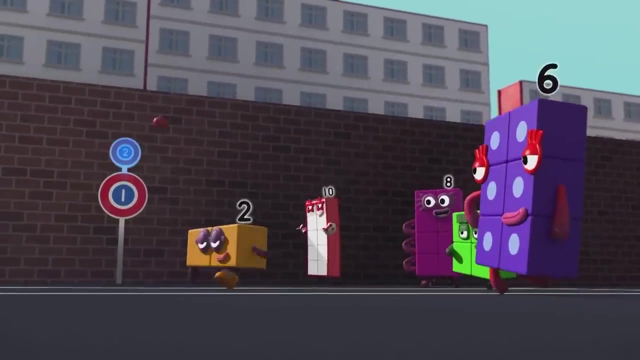 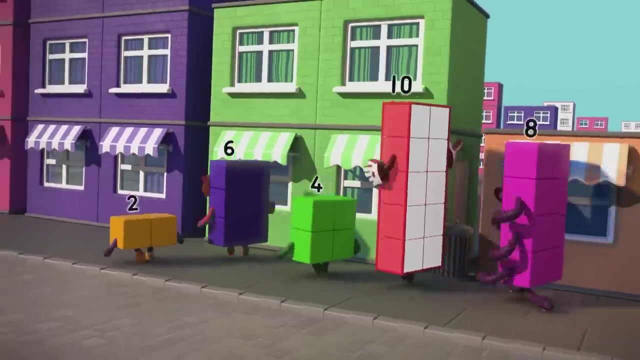 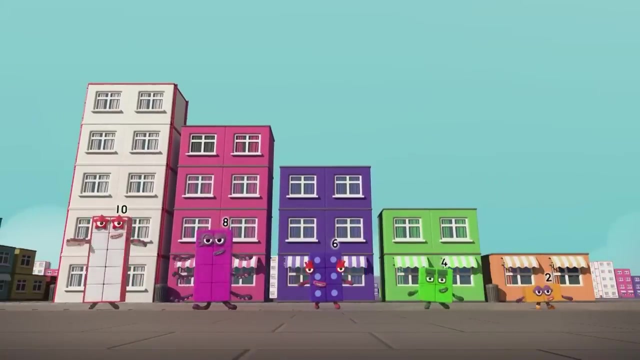 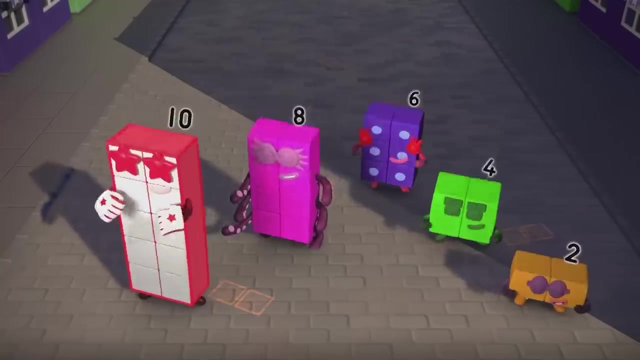 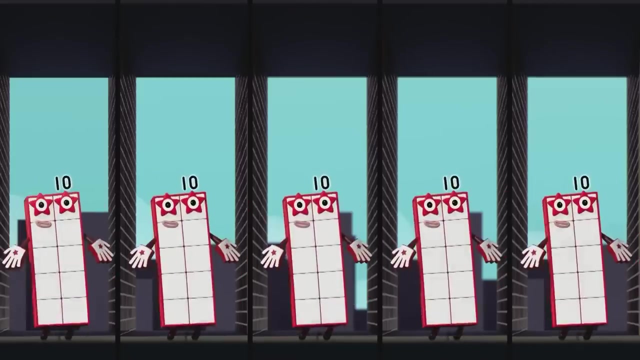 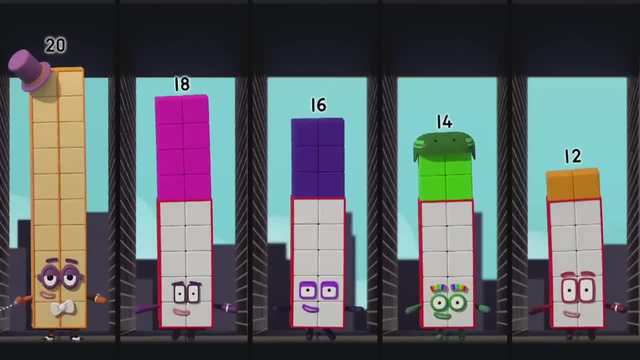 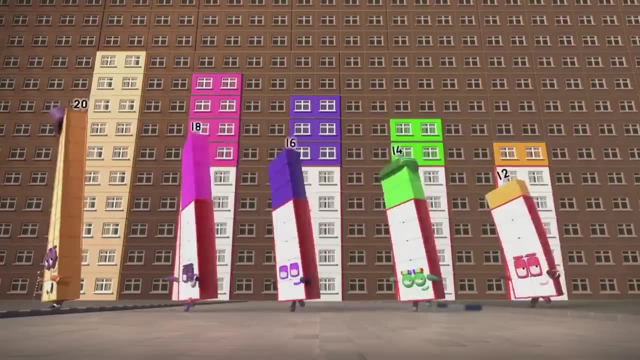 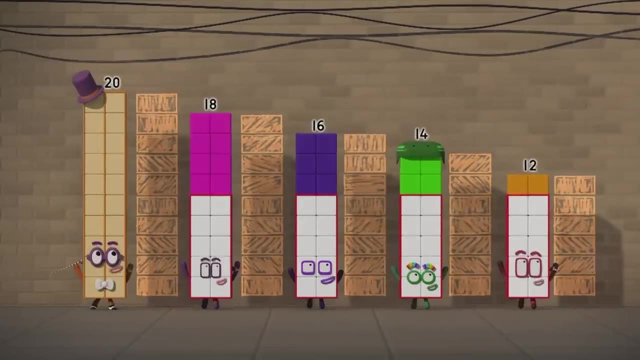 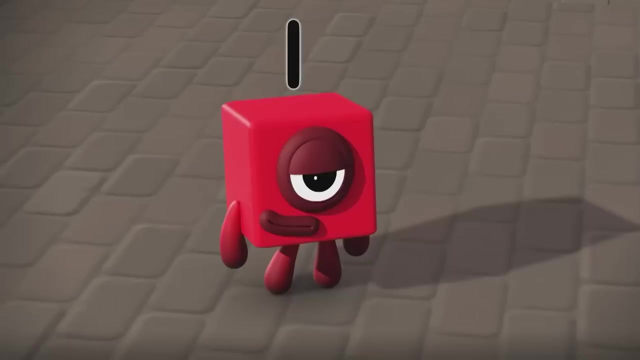 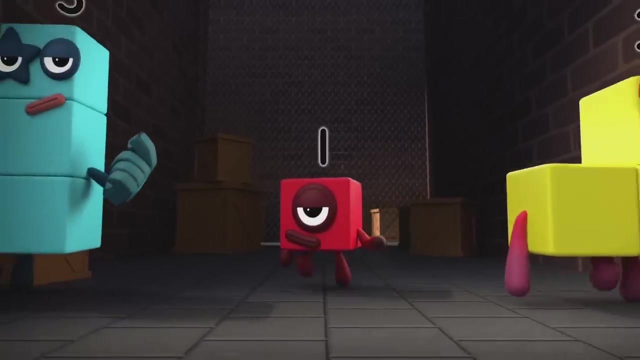 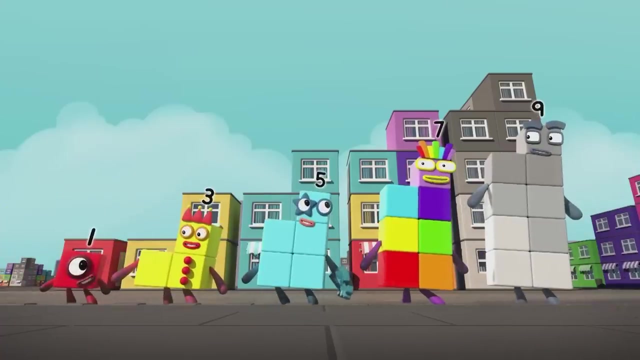 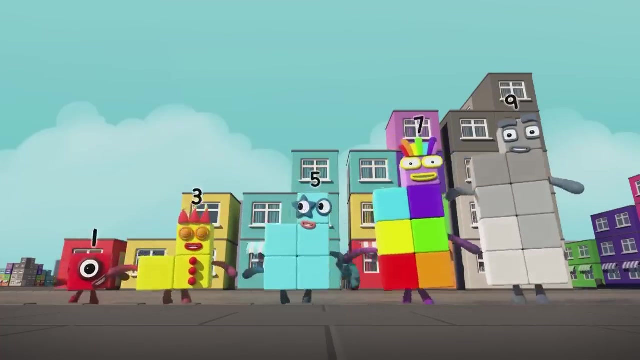 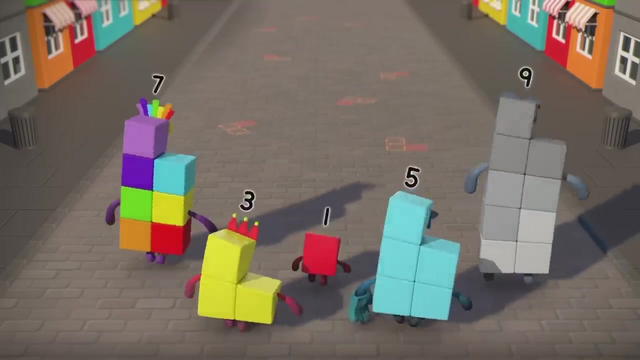 Sixteen, Eighteen, Twenty Evens Even tops Evens Made of twos. Odds Odds One, three, five, seven, nine Odds Odds: Odds Made of twos With a one on top. 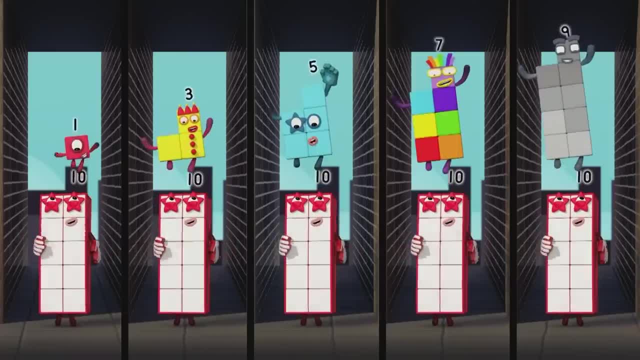 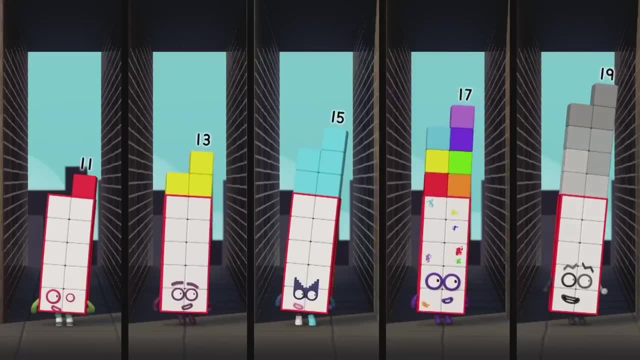 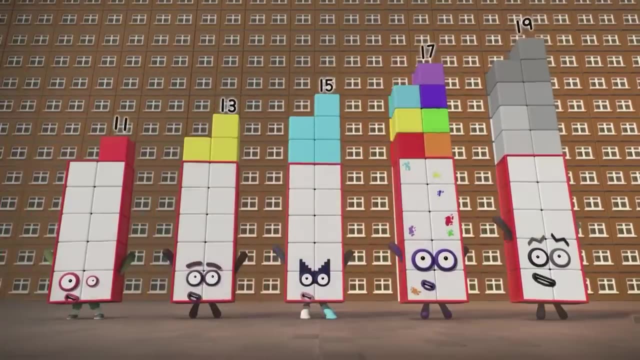 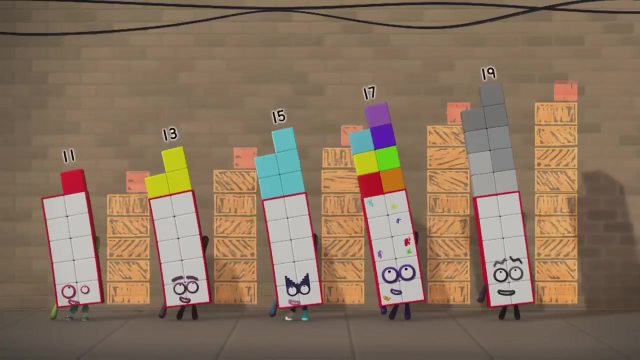 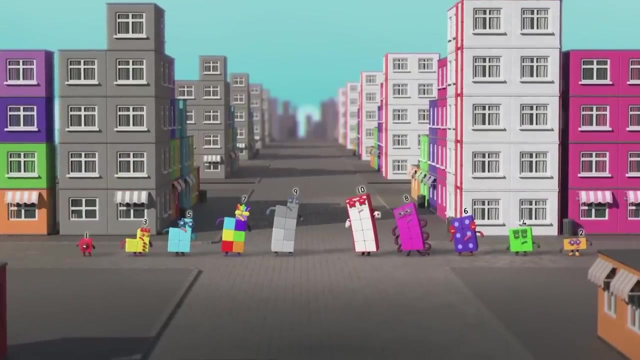 Tens Odds Eleven, Thirteen, Fifteen, Seventeen, Nineteen Odds. Odd blocks. Odds Made of twos With a one on top: Odds Evens Odds Evens Spittins.